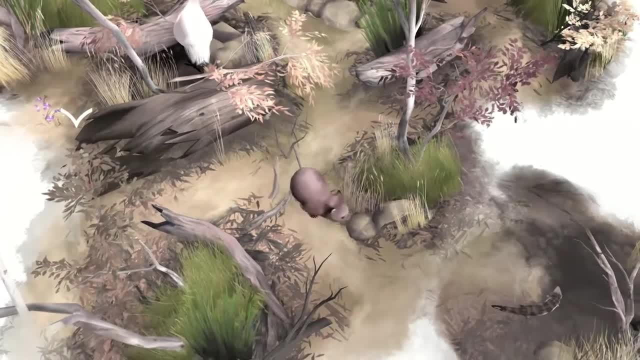 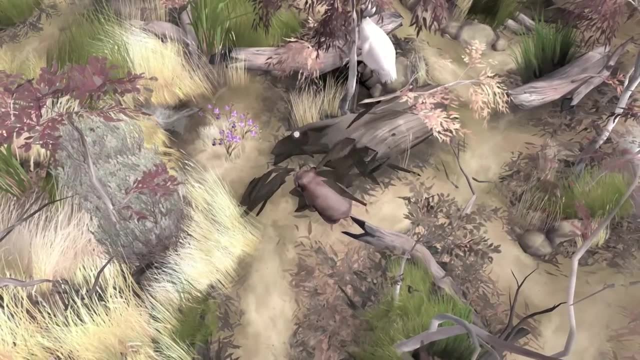 world around it. but then, as you stumble across a wildfire towards the end- and don't worry, there's no big peril involved and there's like no horrible twist- shock ending that kind of painting- the world out around you is flipped on its head because it's smoke and ash all around. 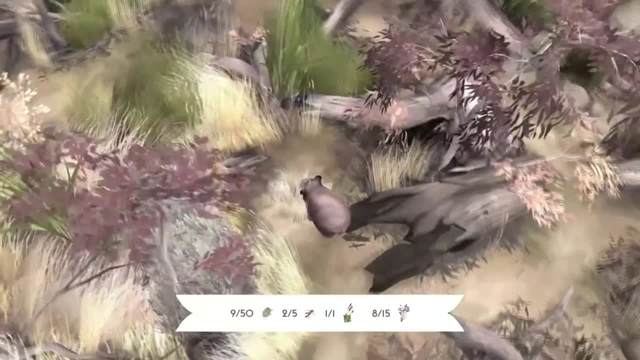 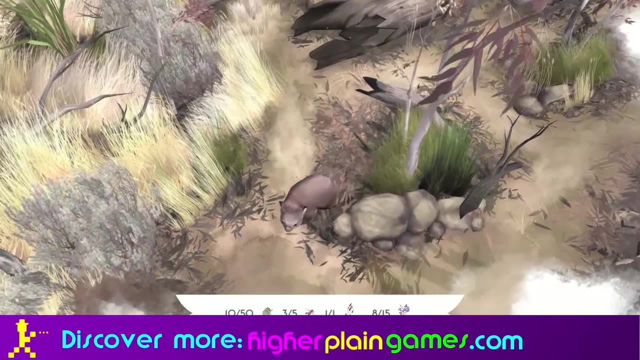 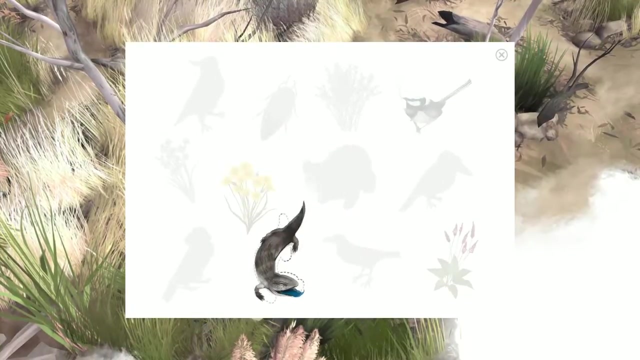 you and you can only see what's in front of you For a little while, which is a really good play on things. The game itself sells its message quite nicely around wildfire and needing to cultivate and look after our wildlife and our wild inhabitants, but it doesn't oversell the message in like a slap you around the face kind of way. 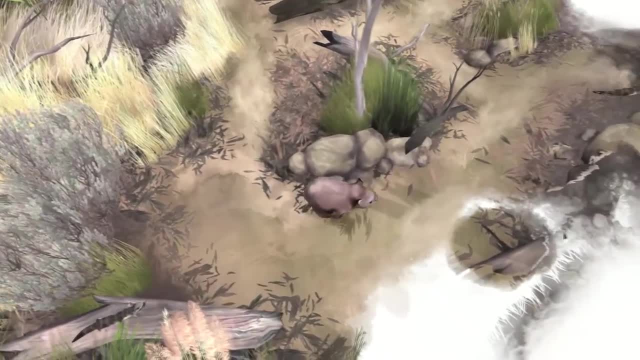 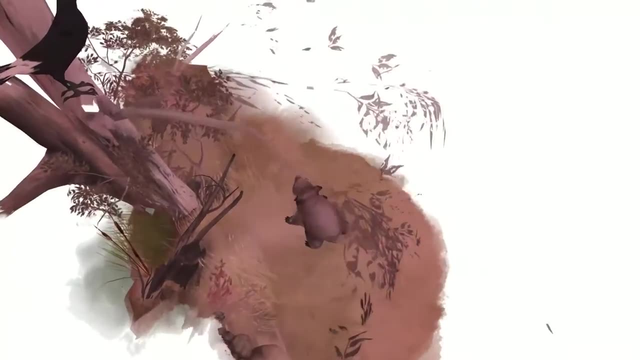 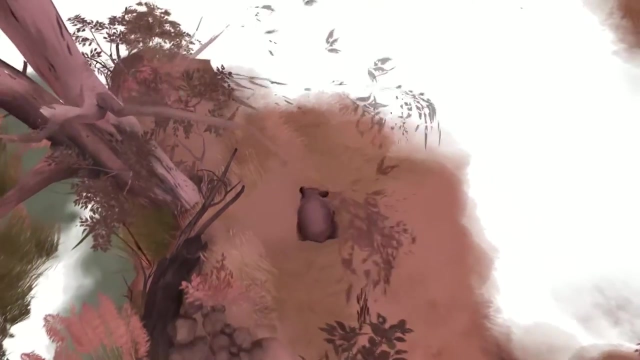 and it serves its story in a way that could be used as a bedtime story to be repeated over and over again. like other kids where they're like, I want to read that story every day. and you're like, really, Because this game can be completed in 30 to 40 minutes. it took me just over 40 and that was. 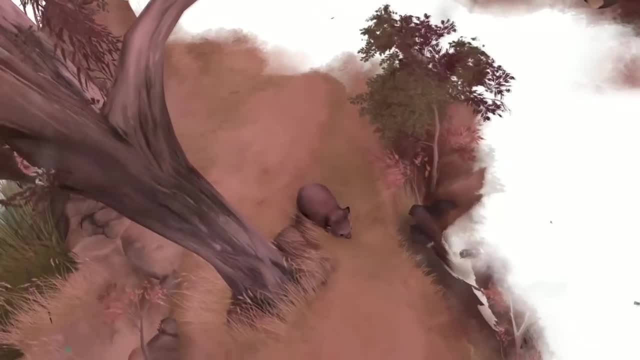 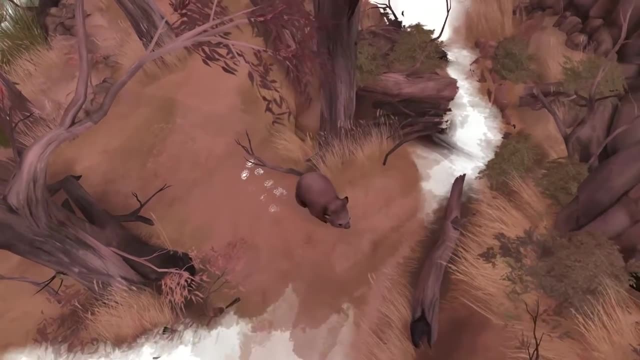 because I was busy trying to get as many of the 100-ish collectibles that you can get as you go through the game. so if you've got a young kid that can't necessarily do all of the clicking in the right areas, then what they can do is point to the animals that you kind of see on your travels. 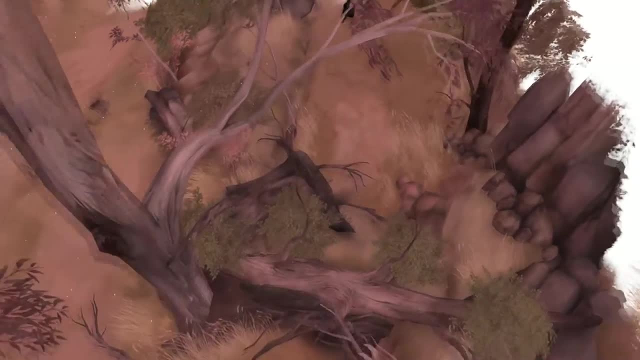 and you'll be able to add them to your collection so that they feel kind of like they're interacting with the game. or if they're happy with the game, they can just click on them and they'll be able to play with it. they can kind of click around on different parts of the map and colour in the world. 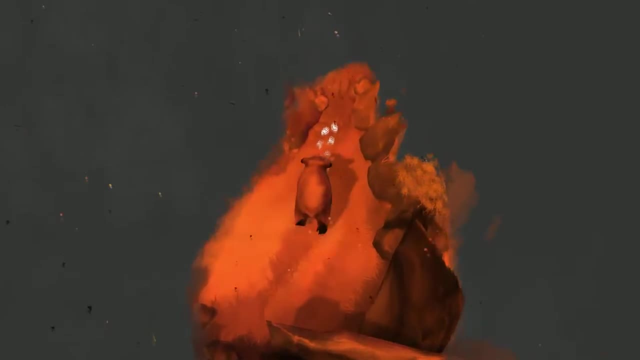 as you go through the story. it's really that lightweight. there's a couple of things that did slightly irk me with the game itself, and that is that when you get into certain areas around, like branches that you would squeeze under or jump over, the game takes over and starts to do it for you. 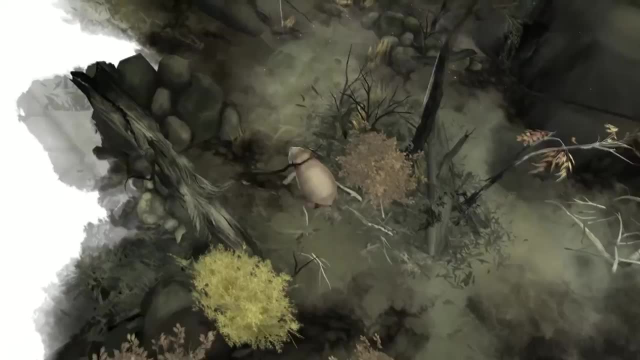 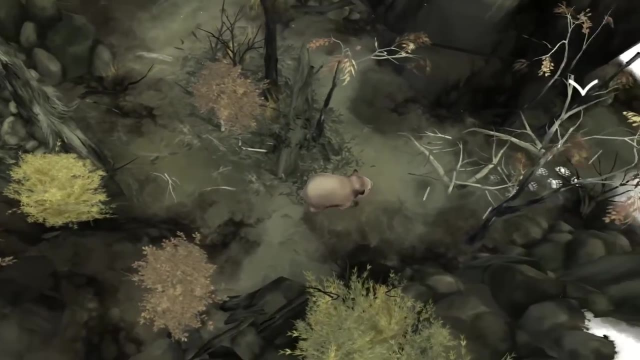 but actually I'd seen a collectible in the corner that I was busy trying to click on to get to, but the game wouldn't. let me kind of go back to get it. so it's very much a Fordmentum thing Style of game and once you cross a path of something it's like a path of no return. so you 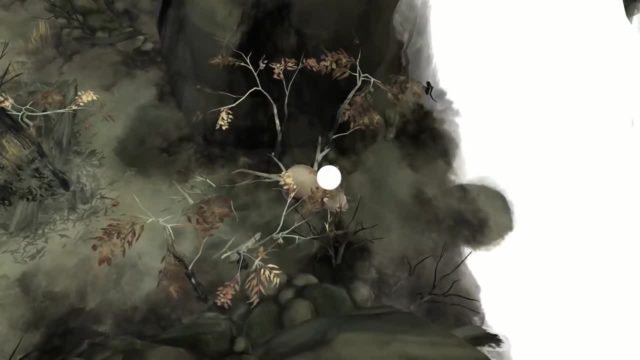 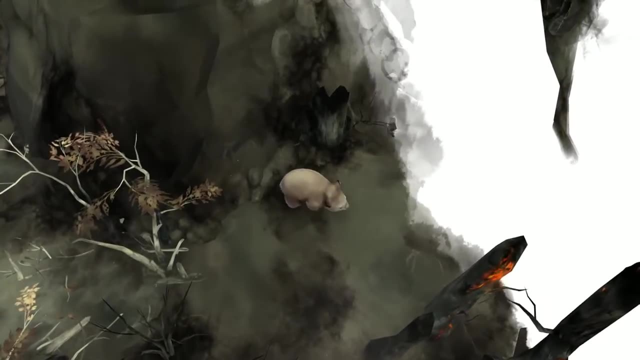 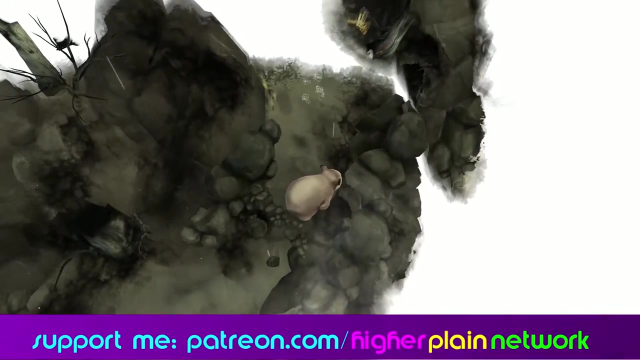 can't go back and grab something, and that, aside from the length, was really my only issues with Paperbark at all. Just a big shout out as well to the soundtrack. I really like the way how the pizzicato strings work throughout all of this game and how it gives a warm, folksy vibe like